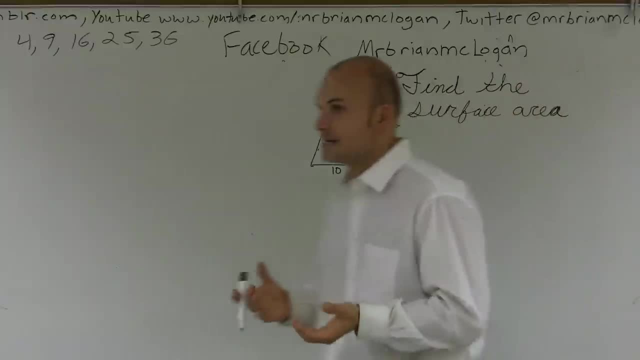 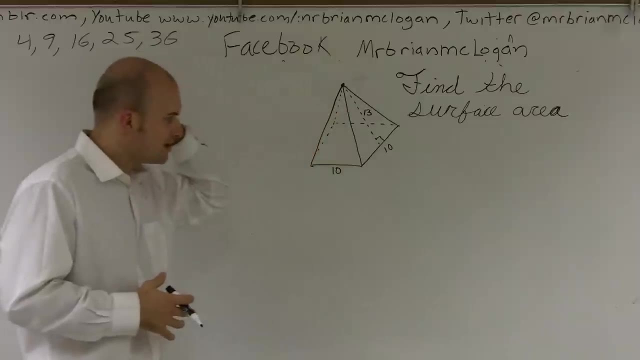 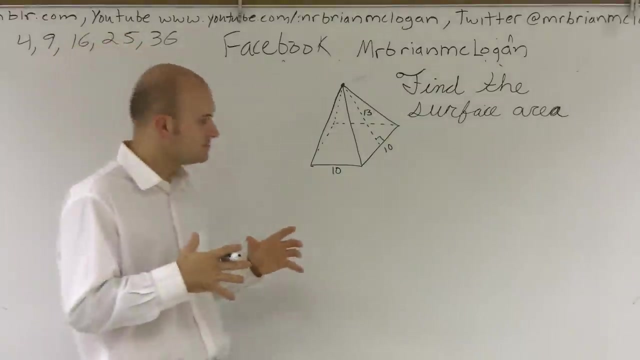 trying to look at different ways for you guys to understand it. So what we have is we have a pyramid here And with this pyramid, what we're going to try to find is we're going to try to find the surface area. So if you guys can always think of the surface area as think, if I 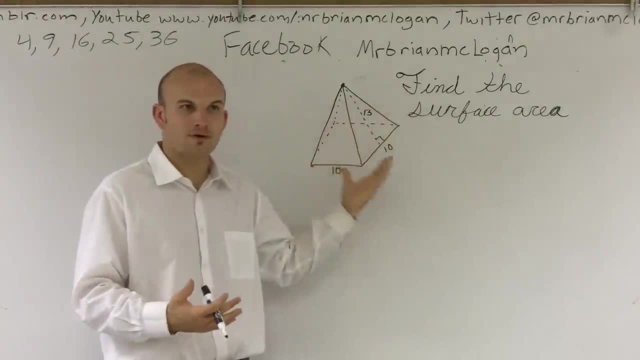 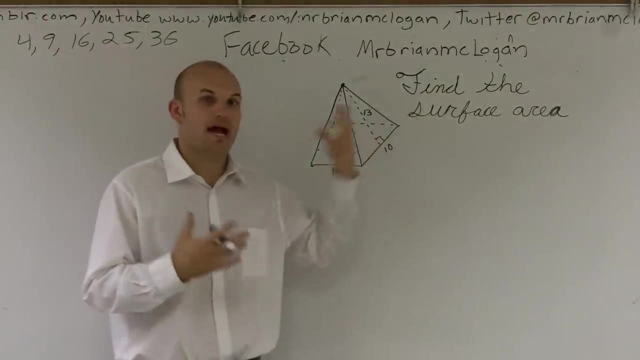 had to paint something, I would need to make sure I covered the whole surface of the whole thing. Or let's say this was, let's say I was going to drop this in water. The surface area would be everything that gets wet. Nothing in the inside is going to get wet, but everything on the outside. 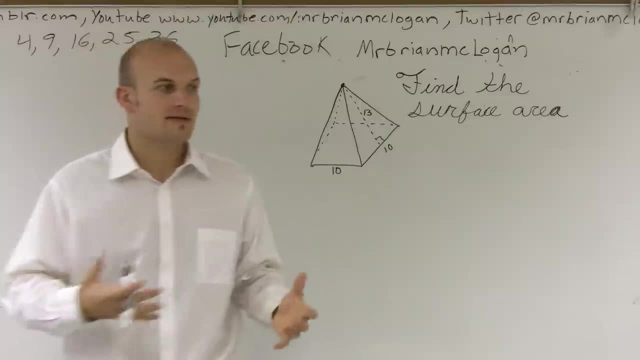 would be wet, So we need to figure out how to do that. So what we're going to do is we're going to figure out what is all this area that is covering up this pyramid. So what I'm going to do is I'm 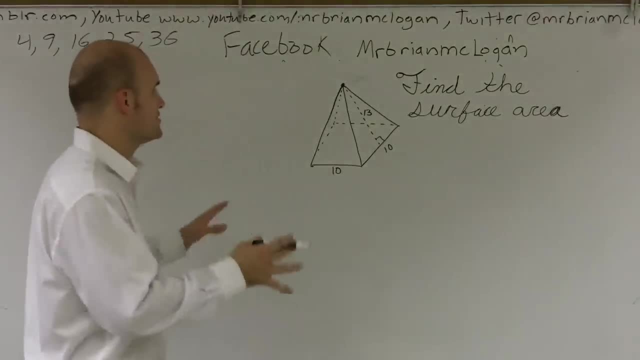 going to make a little net. sometimes we like to say- and I'm going to kind of branch off this onto a two-dimensional- Right now I'm kind of trying to represent it as a 3D- What I'm going to do now. 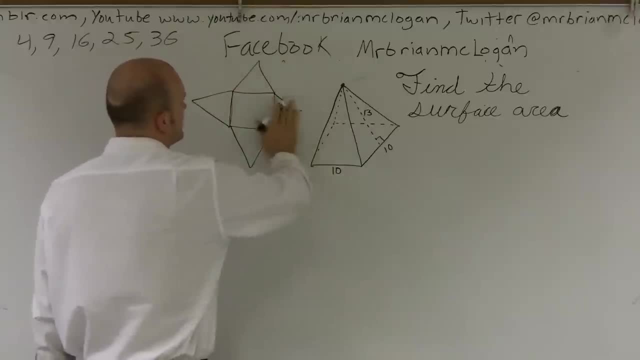 is represent it as a two-dimensional figure, And I know this is really, really bad, but you guys should see if I was doing kind of bring all these sides together and kind of flip it back up to its side, it would look. 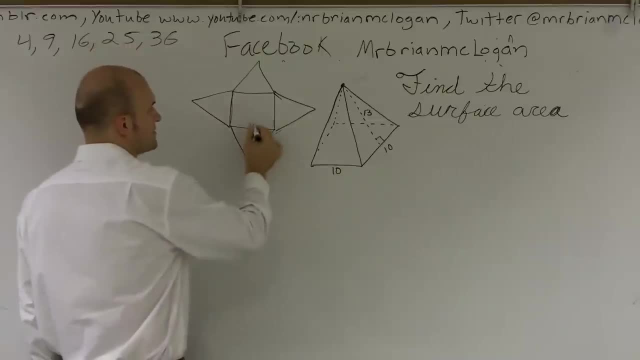 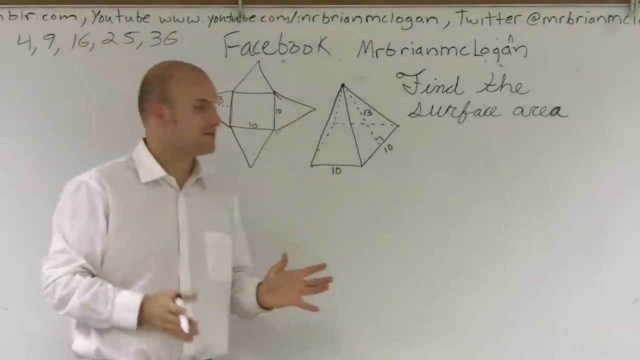 something like this, And what we can notice is, on this two-dimensional, I have a 10 by 10, and then this length or the height of each side triangle is 13.. So when finding the surface area, the best kind of tip I can give you is to break it up and just find every single possible area that you can. 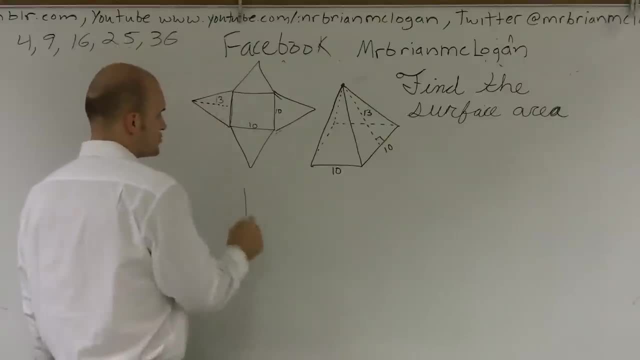 and then at the end, add them up. So what I have is a square plus. let's see, let's call this, let's call this the front, and we'll see, here's going to be the right side, we'll call this the left side, and then here, we'll call this the 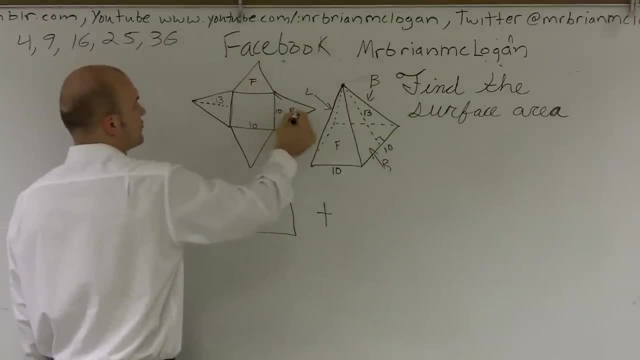 back side. So if I have, this is the front right, no, front right back left. So first one let's do is front which is a 10 by 13,. I think they're all 10 by 13,. yeah, Front plus. we need to do the right side plus. 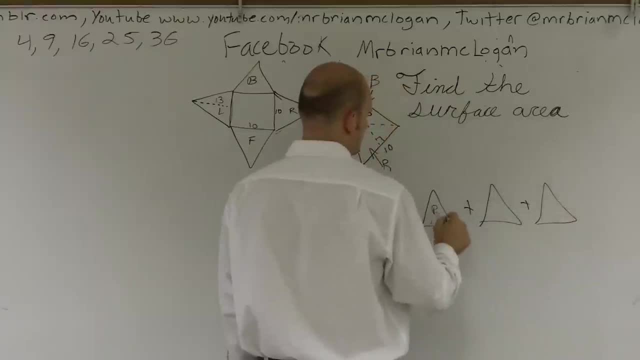 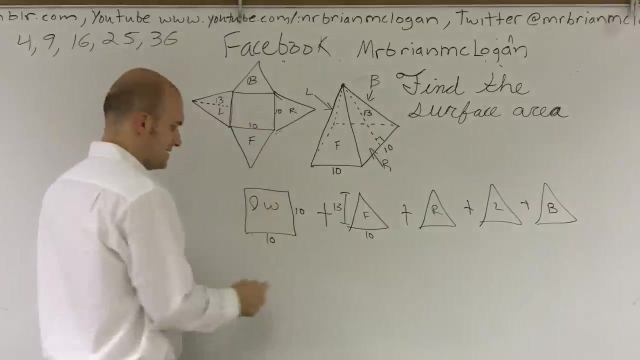 the left side plus the back. So therefore I have all four sides and I have the bottom, the base. So to find the area of a square that's going to be your length times width, 10 times 10 is going to give me 100.. 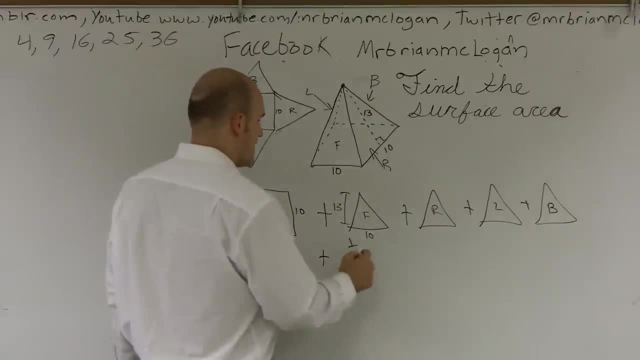 Plus find the area of a triangle That's going to be: 1 half length times width. 10 times 13 is 130.. Divided by 2 is 65.. Plus another 65.. Plus another 65.. Plus another 65.. 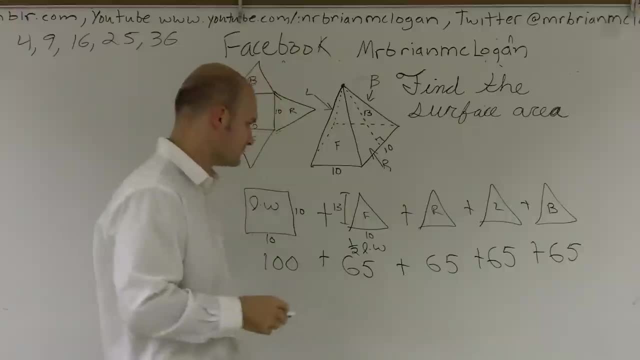 Because each one of those triangles are all the same And when I add these all up, 65 plus 65 is 130. Now I have 260 plus another 100 is going to be 360. And I don't know what it is. but if we are using units, 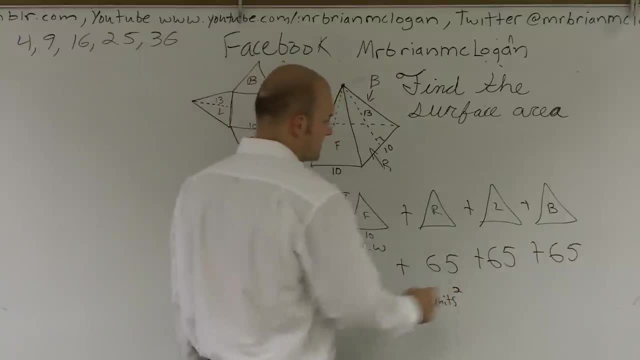 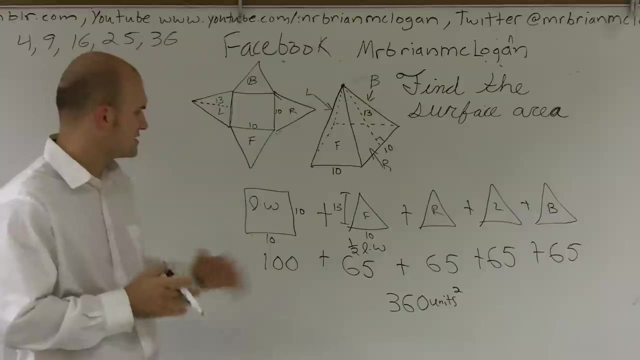 on this problem or not, But one thing: since you're doing with the area, it is going to be a squared unit, So that's just one thing to remember. As far as this, I can't remember the problem. I think I was just using units. 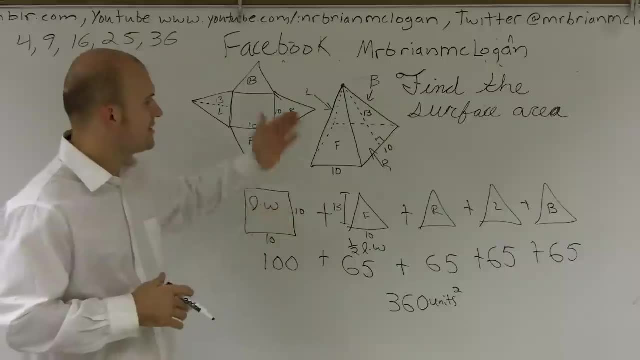 So if you're 360 units, you're going to be using units squared And that's how you find the surface area of a pyramid. 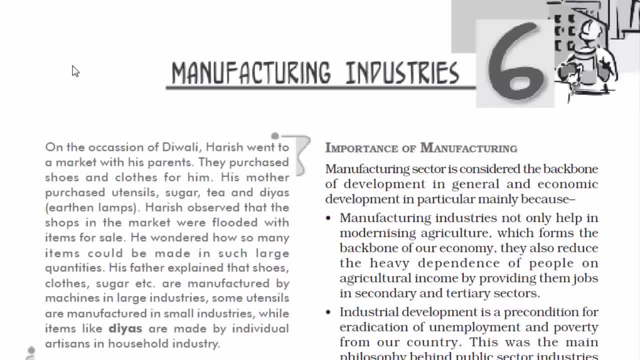 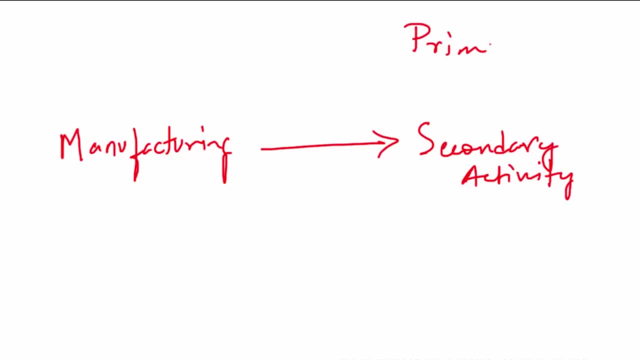 Chapter 6. Manufacturing Industries. So in this chapter we will purely speak about industries that prepares things, that manufacture things. Now, always remember, manufacturing is associated with secondary activity. We have heard about all the different sorts of activities like the primary. 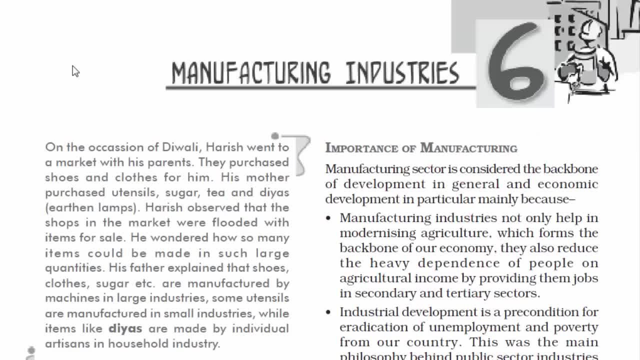 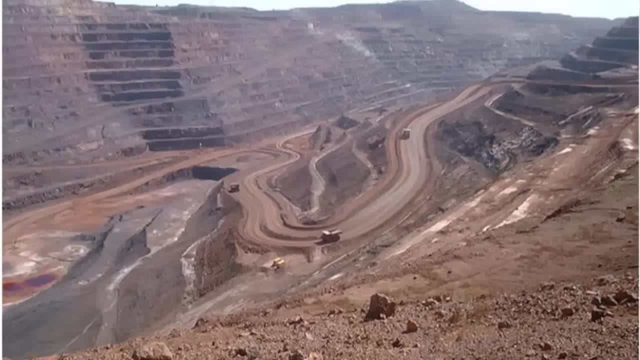 secondary, tertiary and quaternary. So the secondary sector of the economy deals with the finished good. These are sometimes also called as production sector, because they transform raw materials into products or goods. So I hope you're getting what I'm trying to say. Now here's a fine.